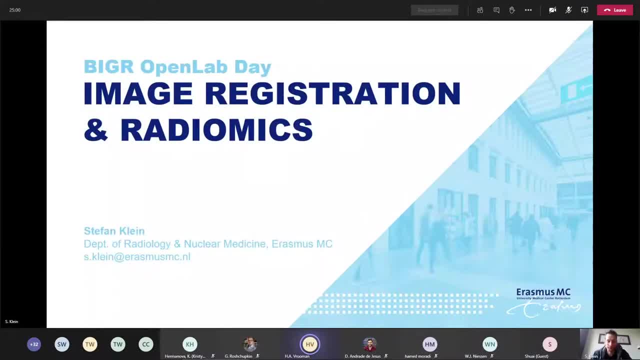 Yes, okay, great. Yeah, thank you for giving me the opportunity to pitch my research. So my name is Stefan Klein, I'm an associate professor in the group and I'm leading a research line on it's called image registration and radiomics, but it's. the topics that I'm working on are pretty broad. 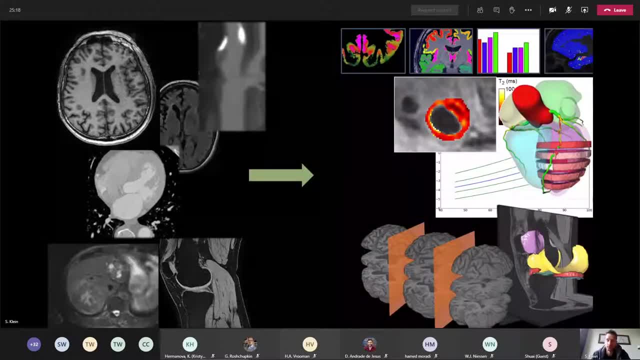 So, in general, the focus of my research is, exactly as Viro already showed, extracting more information out of medical images to, for example, extract quantitative measurements, to do automatic segmentations and compute the volume of a structure, to develop models of anatomy, of healthy anatomy versus diseased anatomy, and really also to go directly from an image to a digital image. 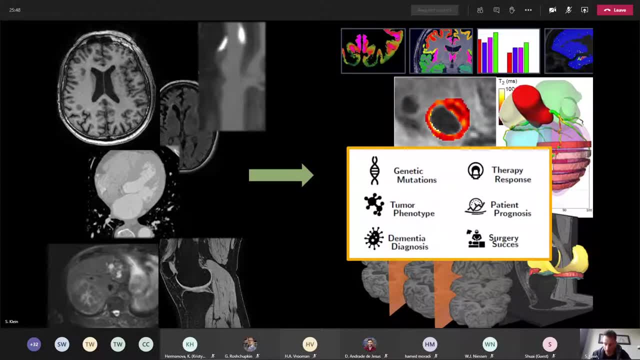 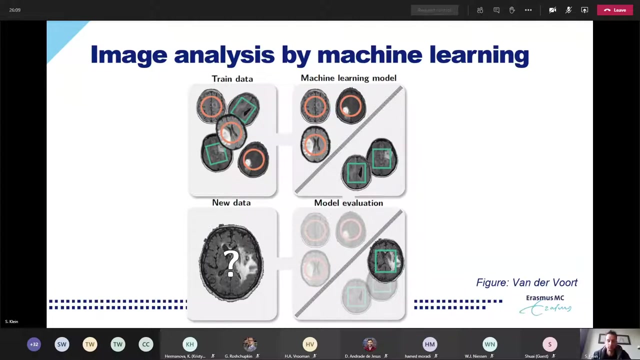 Yeah, a probable diagnosis, or to say something about biological characteristics of a tumor, for example, or just to create nice visualizations. I think it's also an interesting topic. Yeah, for this research we use a lot of machine learning techniques. I think most of you will be somehow familiar with it. 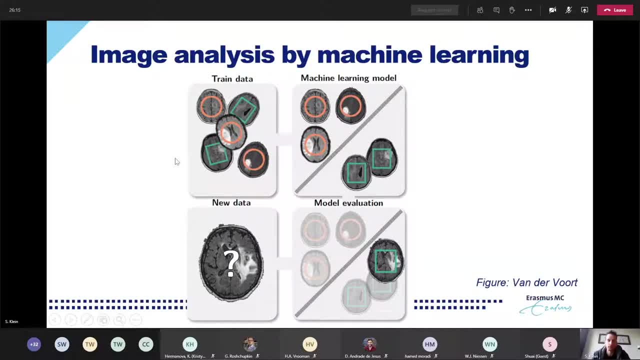 The concept of machine learning is typically that we collect a lot of training data, so a lot of representative images, which are labeled according to the thing that we want to predict. So in this case, we have squares and circles that, in this case, represent two types of tumors in the brain that we want to distinguish based on the MRI appearance. 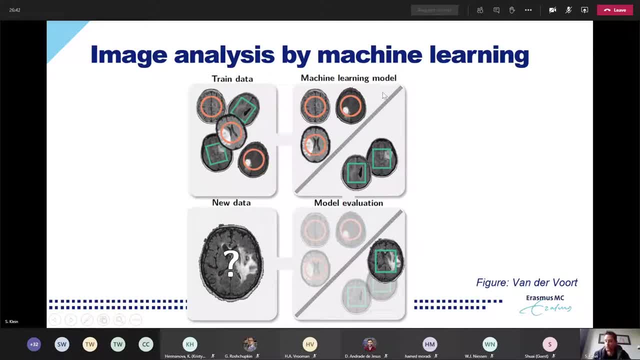 So what we do is we collect a lot of data, then we train a model, a machine learning technique, and there's a lot of variations And models that you can use there and techniques that that's that learns how to distinguish the two classes. 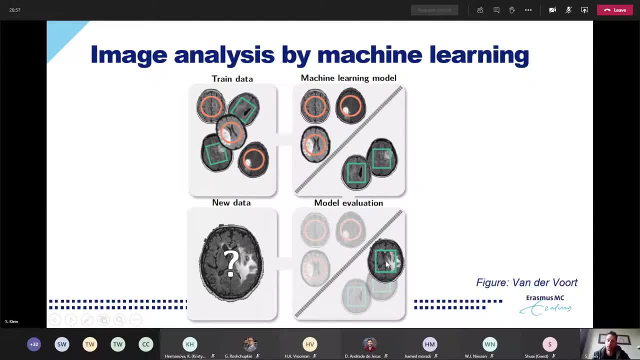 And then for a new example, this model can predict whether it was a square or a circle. So this approach, you see, it's always the same what you need in all applications: First you need a lot of data and then you need some, some tools to train models, etc. 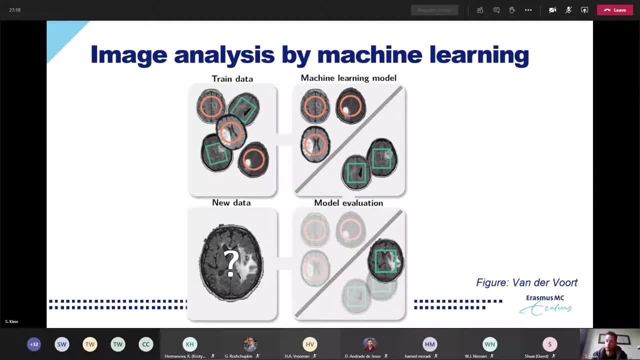 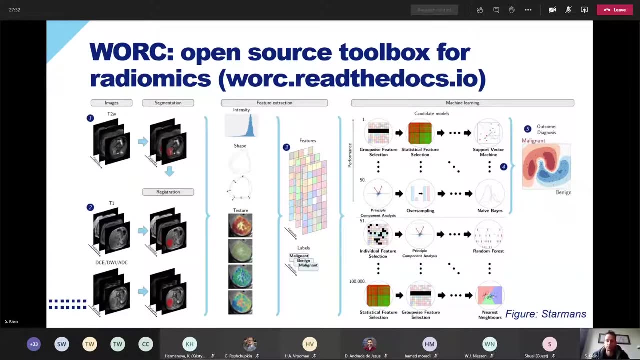 And then you need some, some tools to train models etc. And then you have to test that on another large set of data to see how well your predictions are, how good your predictions are. So to streamline that kind of analysis, we have developed an open source toolbox for this kind of radiomics studies, as we call it. 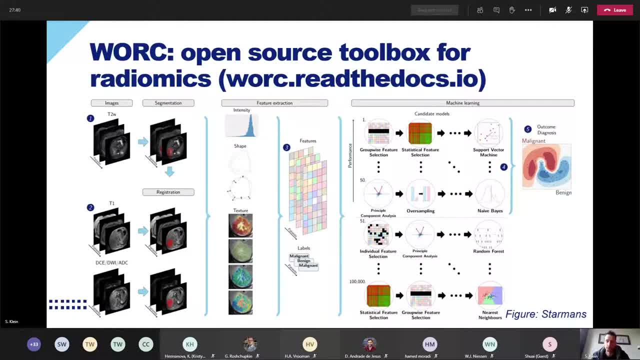 It's called WORC and you can also check here the description online- And that really takes a researcher through the whole process of collecting data, annotating it, computing quantitative features on this data and then fitting machine learning models, And then actually even automatically it compares many different models and takes the best one and then gives you an estimate of how well it performs. 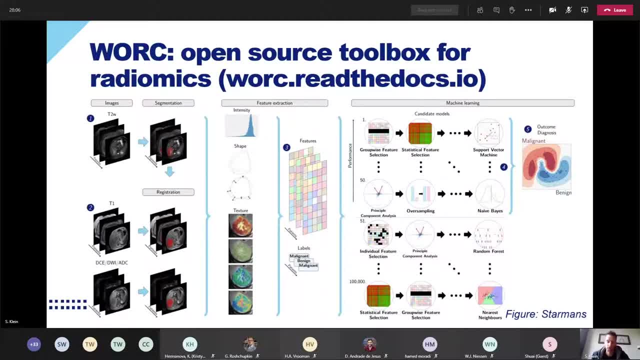 So this was work by Matthijs Starmans, who also proposed some projects. This toolbox We have used a lot in a lot of collaborations within the hospital, but also outside the hospital, And especially it's a very efficient and fast approach. 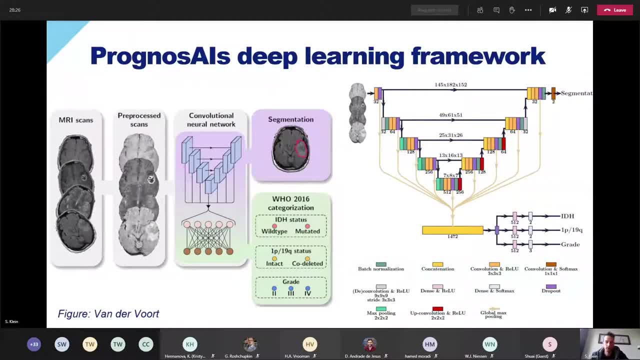 Recently we have developed another framework. This was developed by Sebastian van der Voort. It's another PhD student in my group who are now a postdoc, who also is going to propose some projects. He developed somewhat similar framework, but based on deep learning technology. 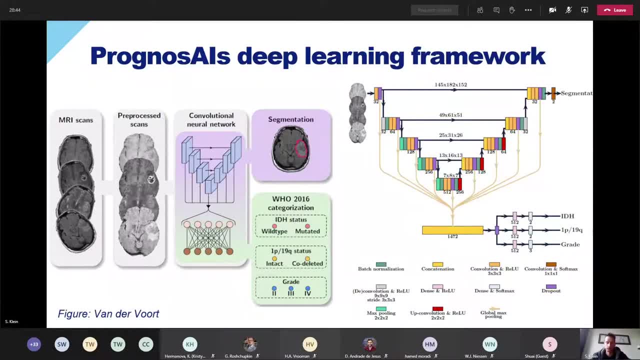 Which is really optimal if you have really large data sets, Whereas the previous framework also works if you have a bit smaller data sets. So he worked on prediction of different brain tumor characteristics And developed a very nice comprehensive framework which also allows you to test different deep learning models. 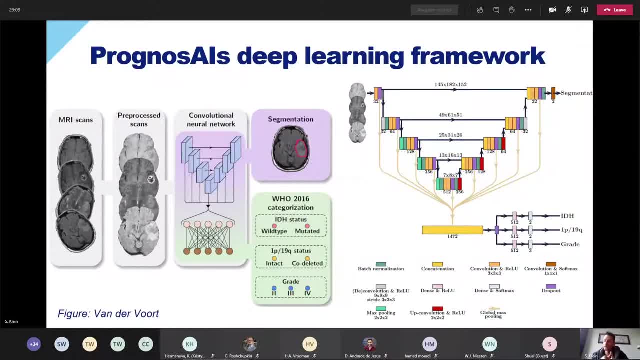 And see what is the best approach for doing either segmentation or predicting some deep learning models. And see what is the best approach for doing either segmentation or predicting some deep learning models. genetic characteristics of these tumors: yeah, with a few lines of code and run that on a. 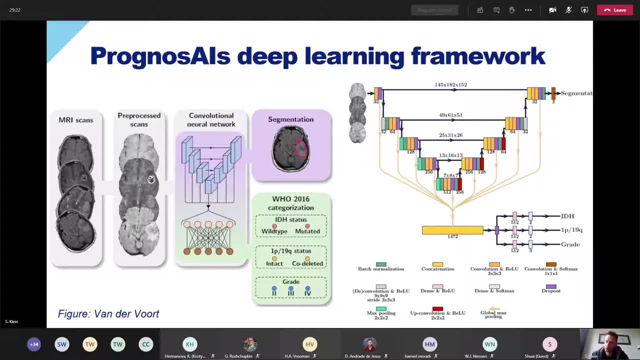 large supercomputer. So also with this framework, I think we will streamline our research in this field, because there's so many applications where this kind of machine learning techniques are useful that, yeah, I don't want to start from scratch in every project.